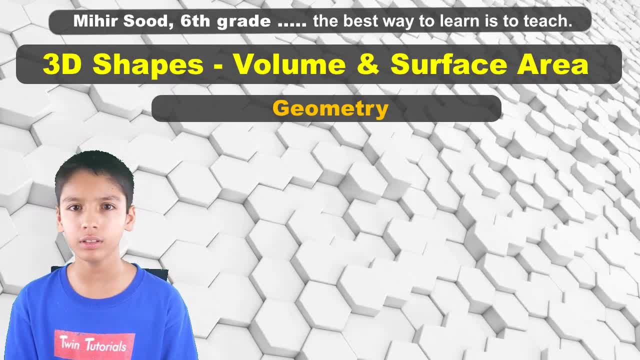 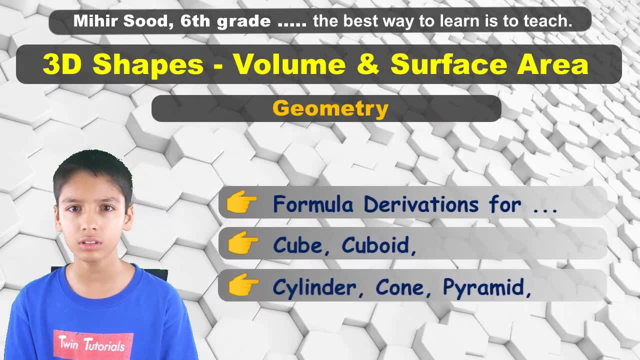 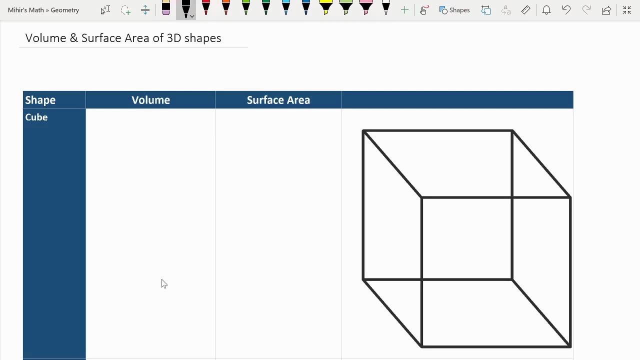 Hello everybody, In this video we're going to be covering the formula derivations for cubes, cuboids, cylinders, cones, pyramids and spheres. So let's get started, Okay. so in this video we're going to be covering the volume and surface area of some common 3D shapes. 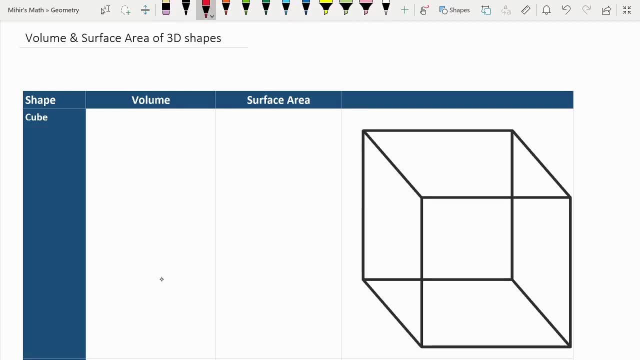 So the first one we have is the cube. So cubes have all equal sides throughout the entire shape. So to calculate the volume we just multiply these two S's together To get the base or whichever other base. Then you would multiply by another S to cover the entire cube. 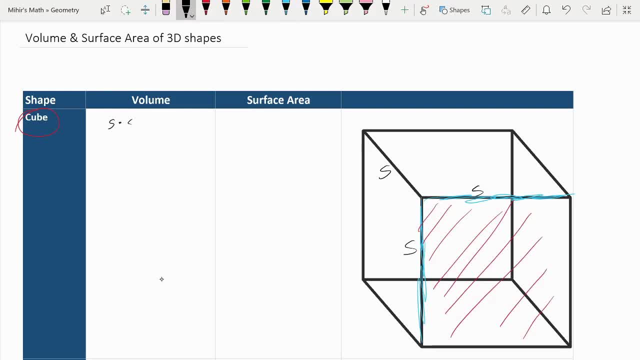 So the volume would just be S times S times S, or V is equal to S cubed. Next, for the surface area. So we would take one of the bases or one of the sides, Which would be all the same because all of the side lengths are the same. 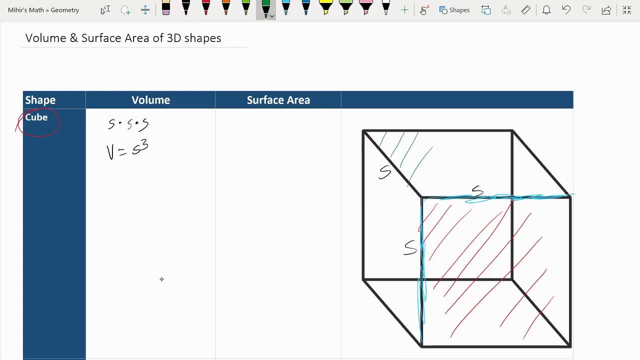 So one side, like the one I'm just going to do in green. So one side would be just S squared And there's six of these sides, so it would be 6S squared. So the surface area is 6S squared. 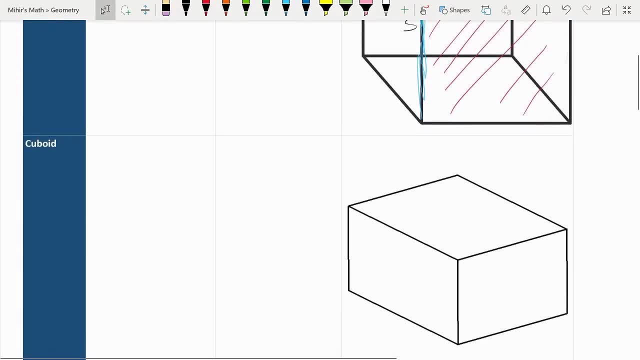 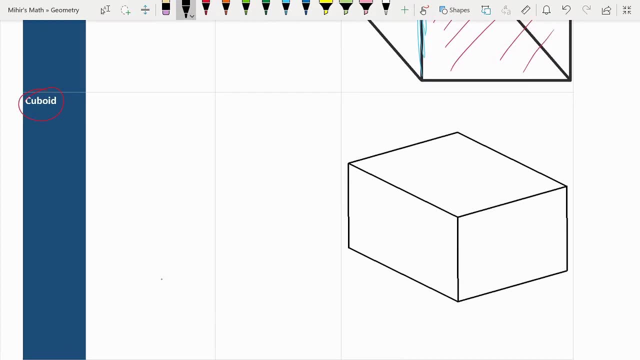 Next, we have a cuboid, So we have a rectangular prism. So to calculate this one, which you also probably know how to do, We would take, we would calculate one of the bases. So in this case, I'm just going to take green side, times a blue side. 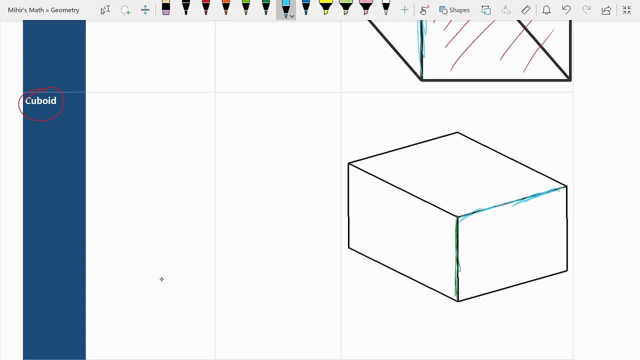 So the blue side, I'm just going to label them. So we'll just call this one blue, This green, here the height. we'll call this blue, here the width, And we'll also get another color, maybe red. 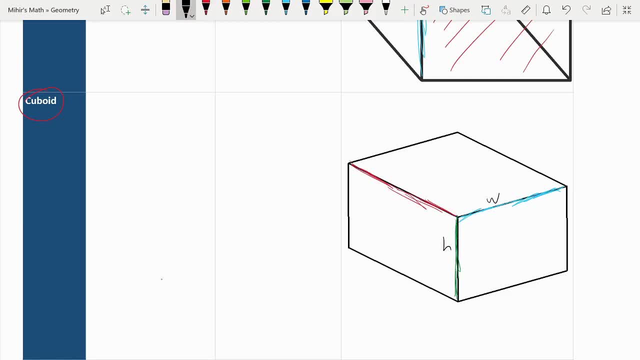 And this I'm going to label as the length. So if you multiply them together you would get the volume. So V is equal to L times W times H, And for the surface area, this one is slightly trickier. 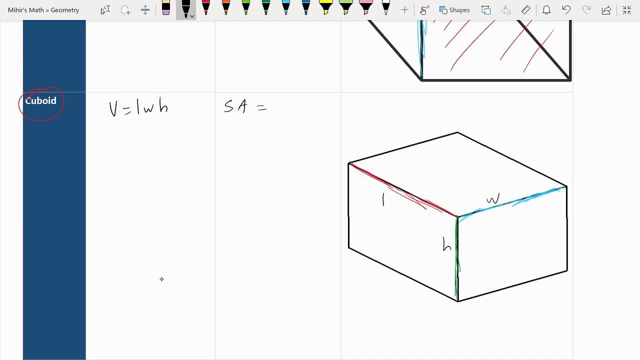 So the surface area. well, if you notice, on any rectangle, in a prism or a cuboid, there's actually two of the same side, going on three times. So for this black side there would be a replica on this other side, on the top side. 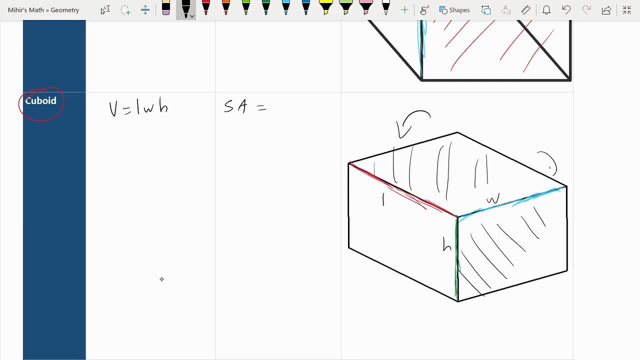 There would be a replica on the bottom side, And for the left side there would be a replica on the right. So we just need to take two times all of those different sides. So the first one would be LW, The next one would be LH. 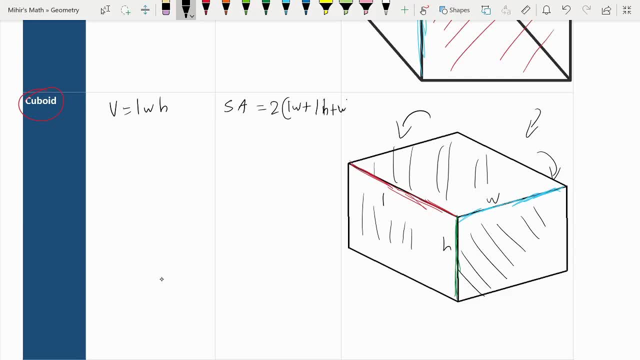 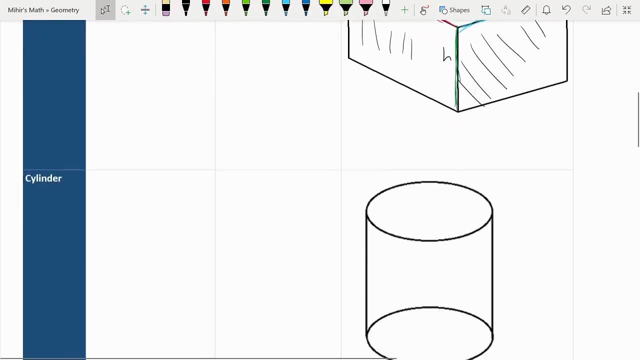 And the next one would be WH. So that would be the surface area of a cuboid or a rectangle in a prism. The next one on the list is a cylinder. So for a cylinder, what we would do is we would calculate the base. 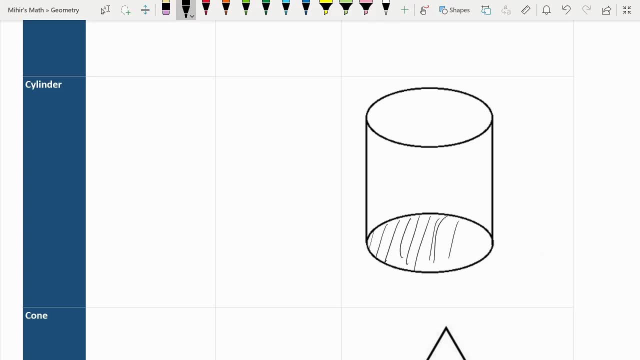 So this base, And we would have to multiply it up by the height to get the entire shape. So the base for a cylinder is a circle, And a circle is just pi r squared, So pi r squared, And then we multiply by the height. 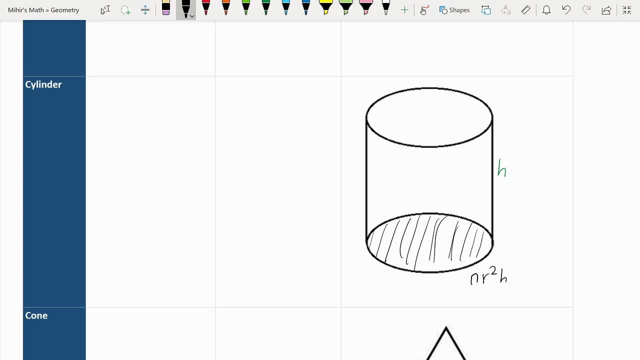 So multiply by the height, So volume is equal to pi r squared times the height. And now for a surface area. So the surface area consists of two circles, So this circle and this circle, As well as this sort of circular shell around this. 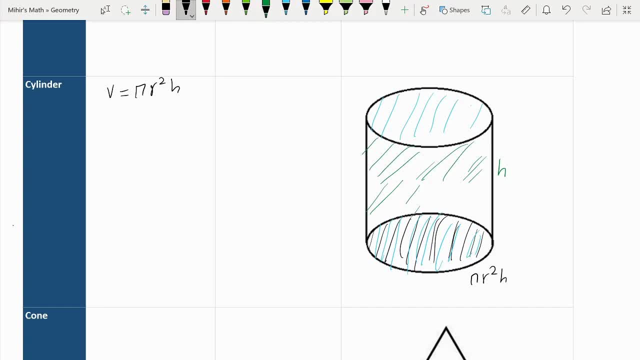 Which I'm going to write in green. So for the two circles we have pi r squared times 2. Because there are two circles And for this sort of outer shell- I guess I'll call it- We would have to add the circumference of the circle. 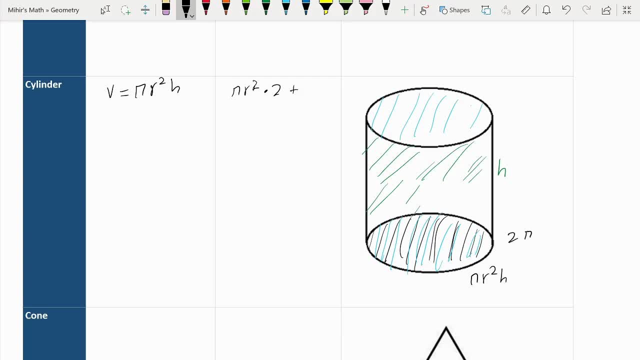 So the circumference of the circle, which is 2 pi r, And we'd have to multiply it up by this height. So we multiply it by its height And if you think about it, it'll sort of get this shell to extend upward throughout the entire cylinder. 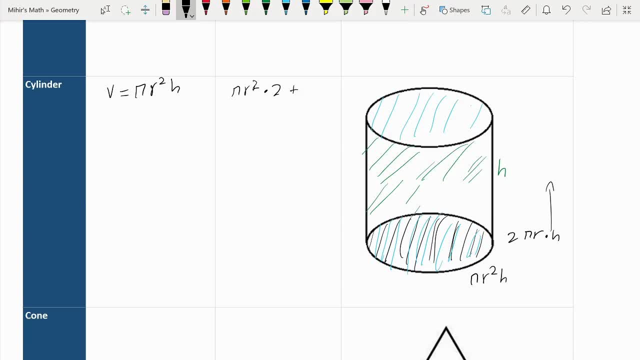 So plus 2 pi r times h. So if you simplify this, You would get 2 pi r squared plus 2 pi r h, And if you were to factor out 2 pi r, You would get the surface area is equal to 2 pi r r plus h. 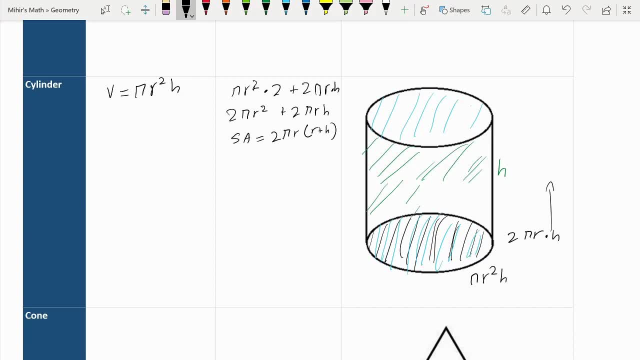 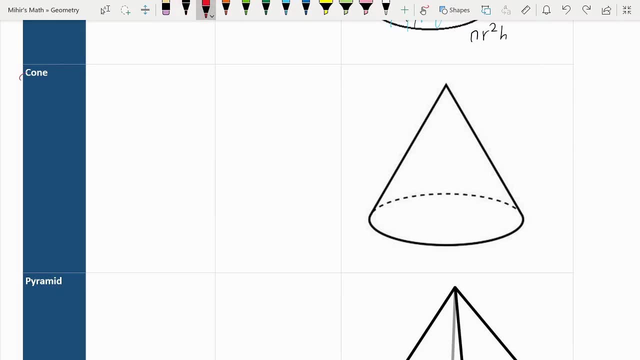 So now let's see how this works. So now let's get into the cone. So I'm going to start off with the volume. So the volume is actually 1 third base times height, And the actual proof for that is in calculus. 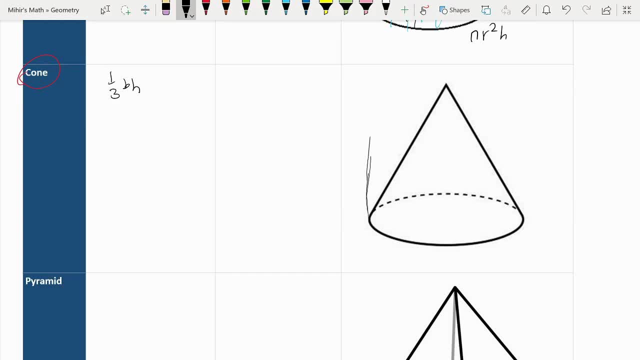 But if you look, If you look at it, If we took this cone And we turned the sides sort of into a cylinder, If you look at it you can actually kind of see that it does look like 1 third of the cylinder. 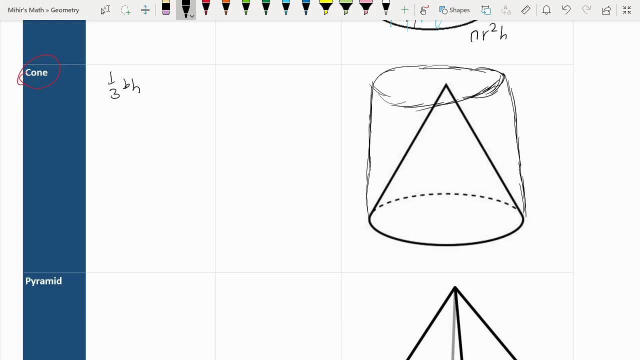 And the base times height is the cylinder And if you look at it, this cone does only take around 1 third of the cylinder. So in this case, for the cone's case, The base is 1 third pi r squared times height. 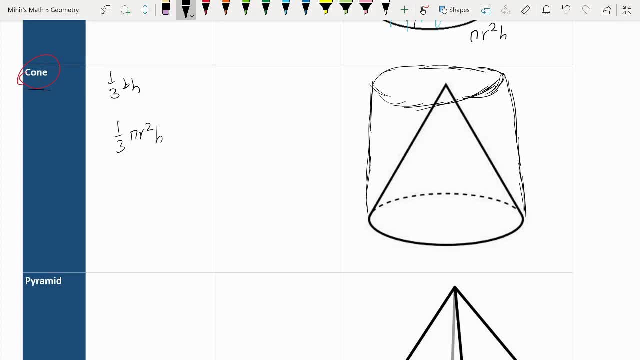 But that is only because it has a circular base and it's a cone. So I'm just going to write v like that. So now we go to the surface area. So I'm just going to label a few of these things. 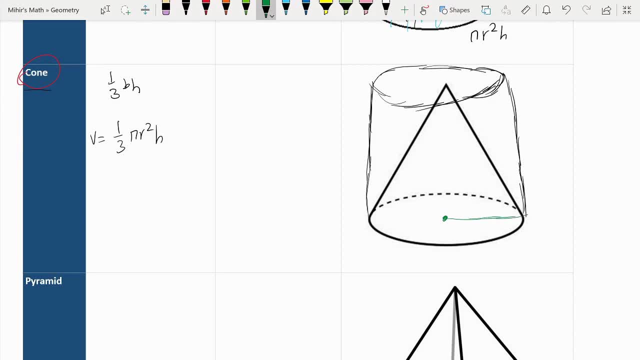 So this would be the radius And this would be the height, And this over here, This is s, This is s for the slant, And there is a 90 degree angle between them. So now we need to get the surface area. 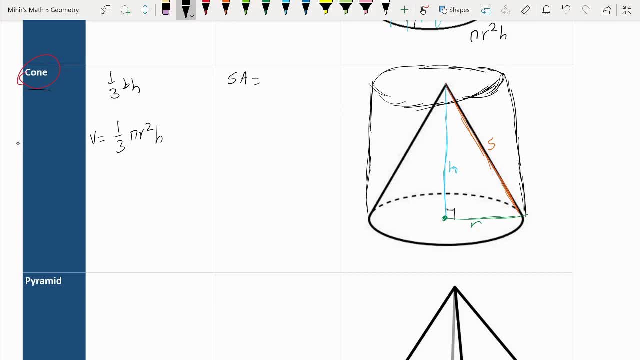 So, along with the volume, the true derivation of this lies within calculus, But this is how much we can do without it. So the first thing would be its base, Which is just pi? r squared, But then we need to get this thing, that sort of coils, up from this base. 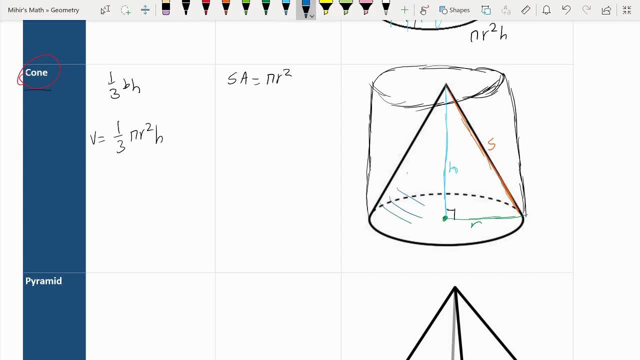 Which I guess I'll label this. So all of this, that sort of coils up from the base. So that is actually, instead of pi r squared, that is actually pi r s, And if you solve this you would get s. a is equal to pi r multiplied by r plus s. 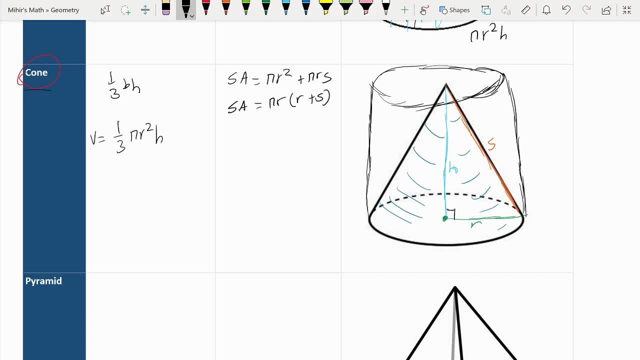 And let's say that you weren't given s, but you still needed to find the surface area. Well, if you look in our diagram, they're actually 90 degrees, Which means we can apply the Pythagorean theorem And we can say that s is equal to square root of h squared plus r squared. 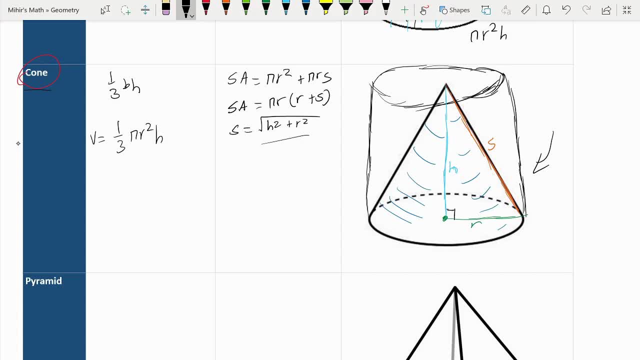 And you can fill this in for the value of s, in case it wasn't given to you. And you can say: s a is equal to pi r r plus square root. So we can say that s is equal to h squared, r squared. 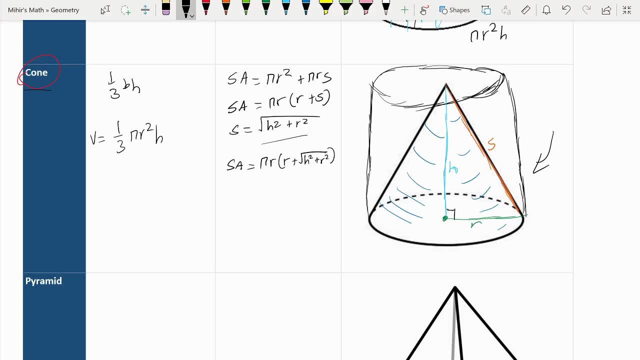 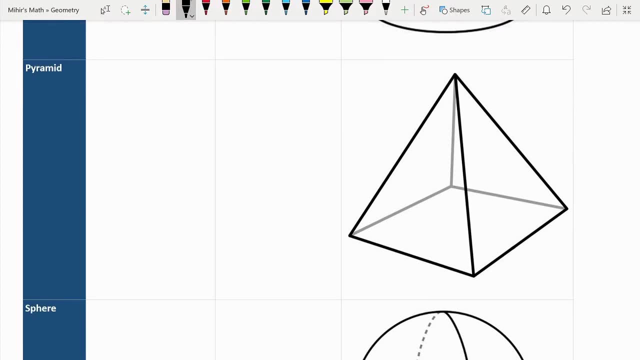 In parentheses like that. So next we move on to the pyramid And this is pretty much the same as the cone. The volume for this is one third of pi r squared third base times height, because this is also a fixture, that sort of cones in. 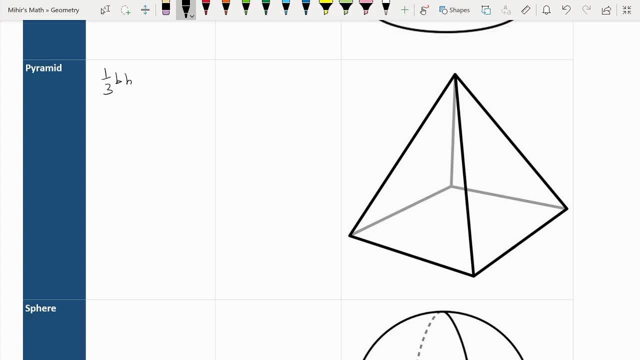 uniformly from the base and if we do the same thing as we did to the cone where we drew a cylinder, if you were to sort of visualize it and draw points upward. my drawing is not the greatest, but I will try my best to show you how it looks. 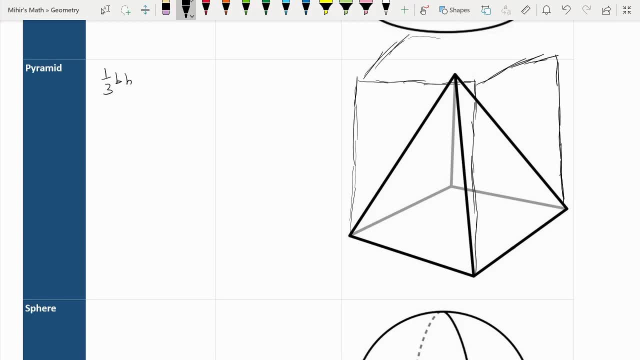 if you did, you can see this does kind of look like one third the full thing, which is a good trick to remember the formula. so now if I were to label these lengths, and with that means that volume equal to one third LW for the base multiplied by the height. so next we have the surface area. 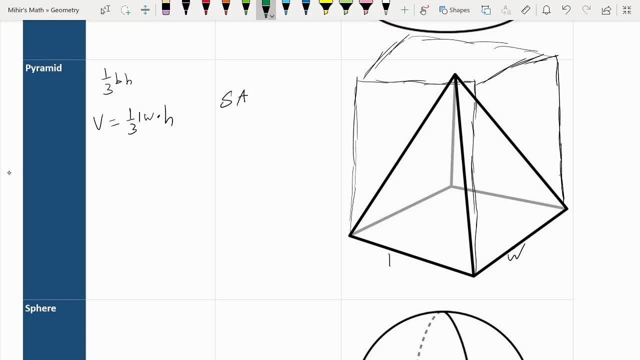 and to solve this I'm just going to label our height here as light. so the surface area first. we're going to do the base, so that's just LW. then we need to add up all of these triangles. so, since it's a rectangular pyramid, there are two sets. 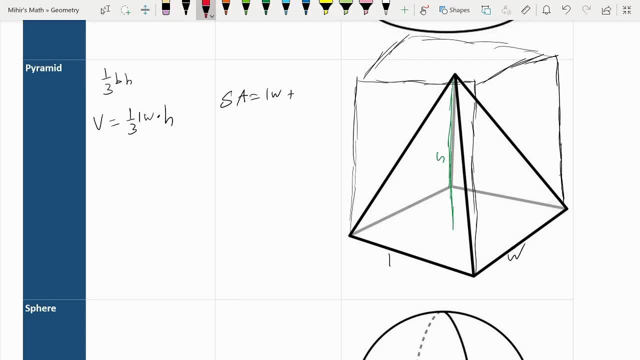 of triangles that are the same. so the first one is: uses this slant here, which I'm going to call, I guess, s1, and then this slant here which I'll call s2, and this would be mirrored on the other two sides. so if you were to solve this and 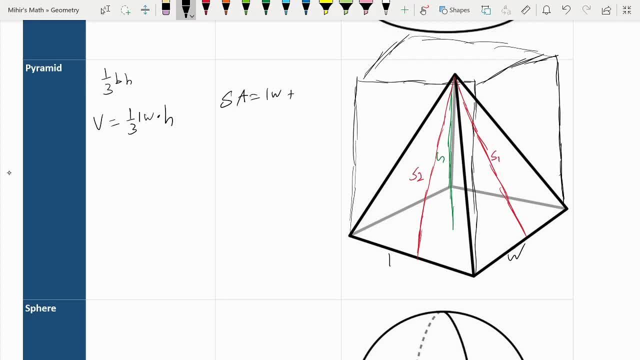 you knew those two slants, then we could simply say LW plus Lvious L times s2.. See, I'm going to write this in a new line, S2.. So the first one would be L times s2, times 1 half, and then there's two of these, so times 2.. 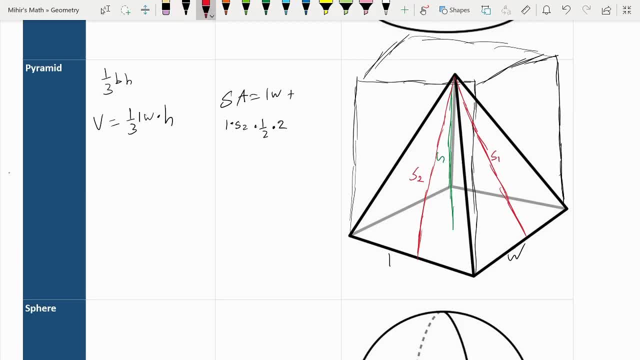 So these two cancel out and we're left with just L times s2.. We also have s1, so W times s1 times 1 half times 2.. These two cancel L times: s1 times 1 half times 2.. 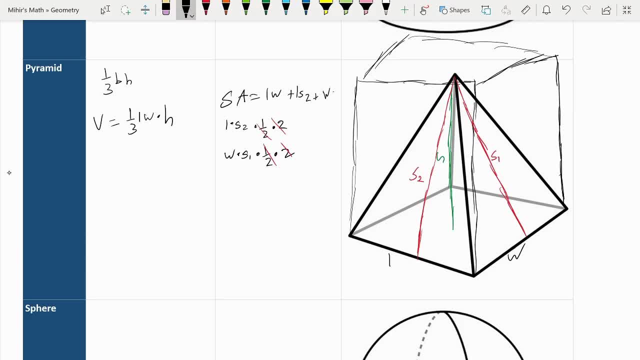 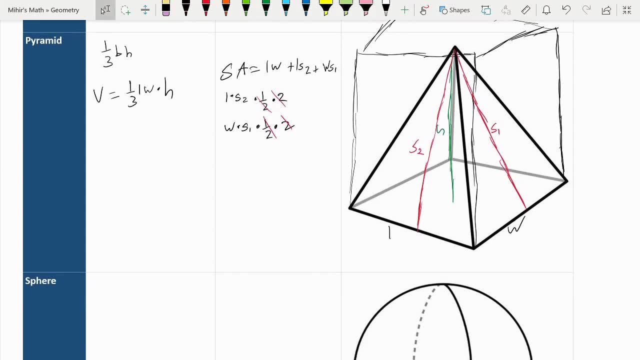 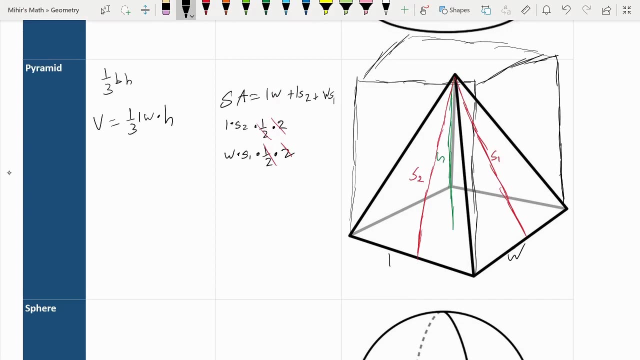 L times s1 times 1, half times 2.. And we're left with plus W times s1.. So now we're left with this scenario, in which case we weren't actually given s1 and s2, and we need to solve for them. 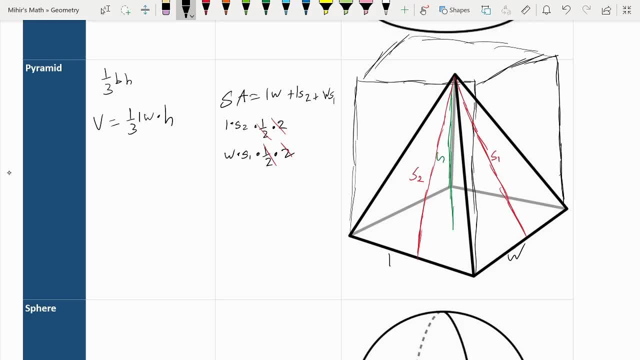 So let's solve for s1 first. So if we weren't given s1, s1 can be looked at as the hypotenuse of a right triangle like this. So one side of it is this h, one side of it is h over there and the other side of it would be 1 half of this. 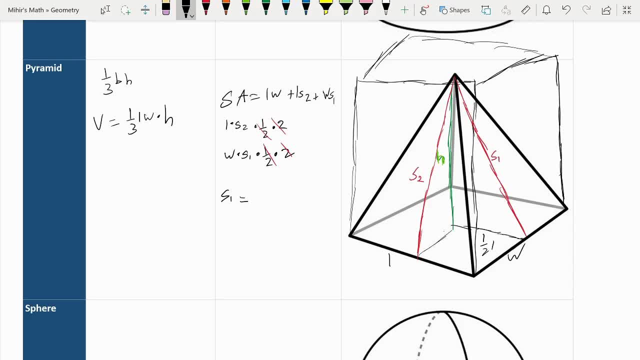 So if we were to solve for s1 here using the Pythagorean theorem, that's equal to 1 half of L. So I'm going to write L by 2 squared plus h squared And a square root And a square root like that. 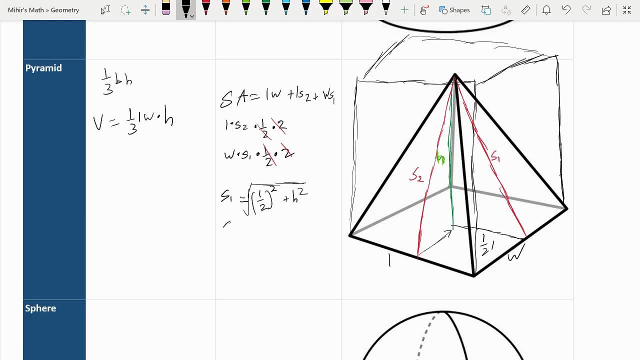 So that's s1.. And for s2, we do the exact same thing. So for s2, s2 is the hypotenuse of this right triangle, with h as one side and 1 half of W as the other side. 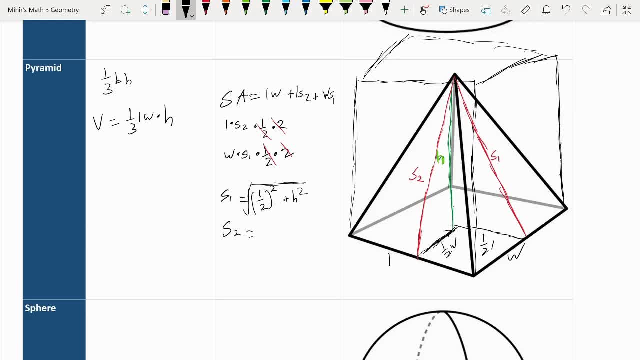 So s2 is equal to the square root of W by 2 squared plus h squared. So if you didn't know s1 and s2, you can substitute these values in for s1 and s2.. So if I try to write it, 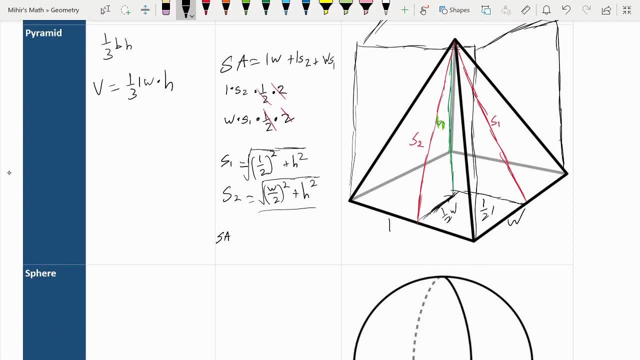 sA is equal to LW plus L multiplied by the square root, And a square root Of W by 2 squared plus h squared. And then we do plus, And I don't have enough room here, so I'm just going to write that. 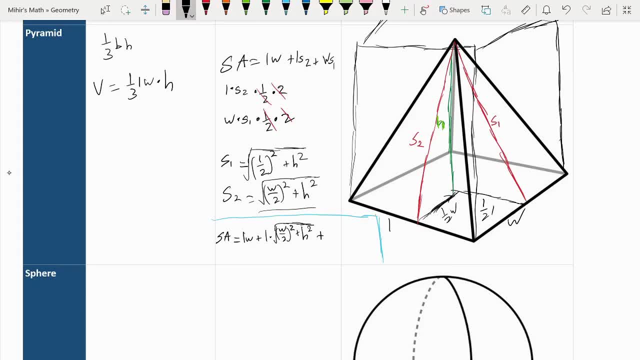 So plus We have W And a square root Of L by 2 squared plus h squared. So if you didn't know the slants, this would be the full, extensive formula of doing it. Of course, you probably can't remember this, so you can just: 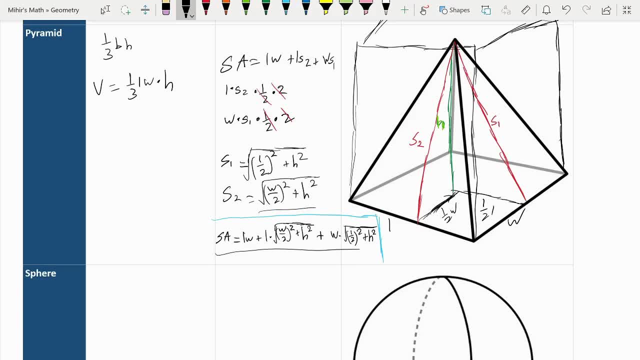 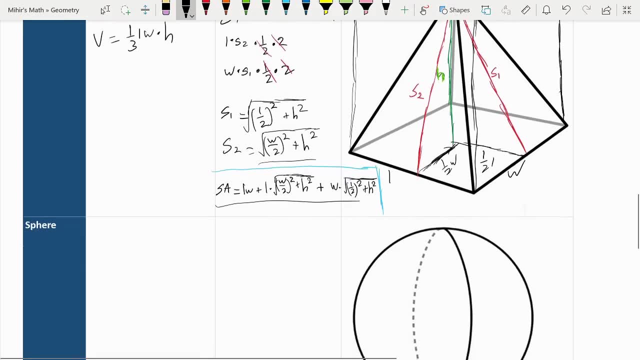 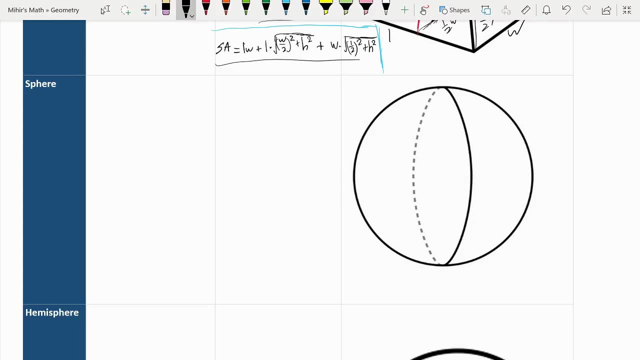 literally find out all of the triangles here using the slants and then just add the base at the end. So that's an easy way of remembering this instead of using the formula. So, moving on to a sphere, I'm just going to cover the surface area first. 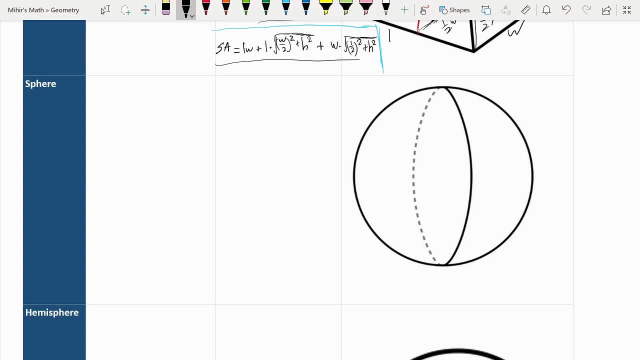 And the true derivation of this is again through calculus, But this is how you can sort of think your way through it, So. So if you had one circle of the biggest section in the sphere, this would of course be pi r-squared. 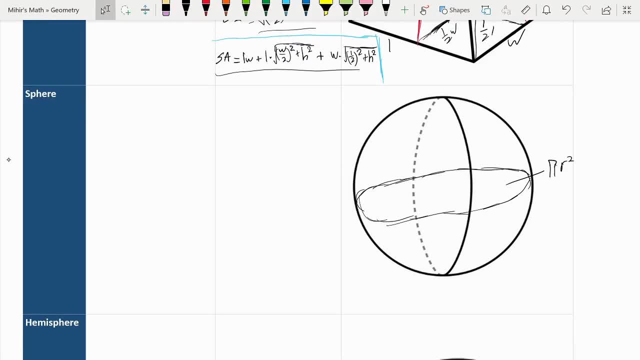 So if you were to sort of look at it, you can see that it would take four of these circles to cover the whole thing And the surface area is 4 pi r-squared. SA is equal to 4 pi r-squared. 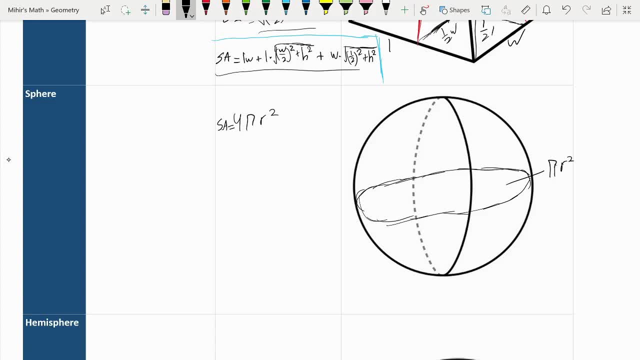 And you can see that it would take like four of these circles to cover the whole thing. So next we have our volume. So for the volume of the sphere, I'm just going to get rid of this, so I have an open canvas. 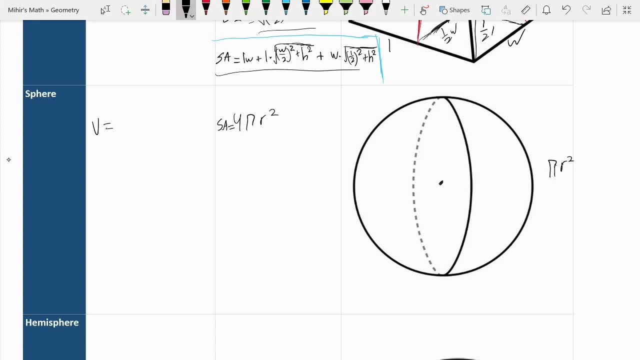 So for the volume of the sphere, if I had sort of cones lining the outside of the sphere like this- and we had a lot of these cones- I would have had more cones making the entire sphere. So I had way more of these cones. 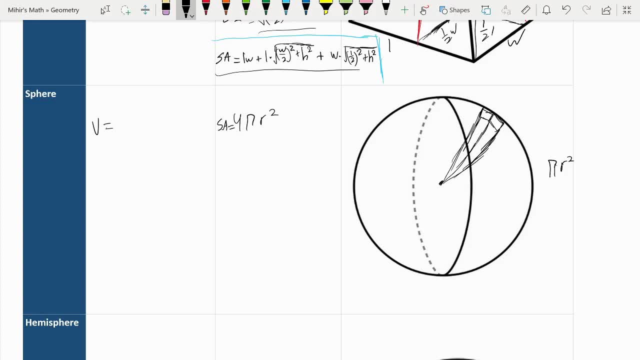 So obviously, to make this actually in a spherical shape, we would need to continue this pattern until these bases, these bases here, were infinitesimally small, Really, really, really tiny, And that would eventually create a perfect sphere. So if we were to write that the formula for all of these cones- 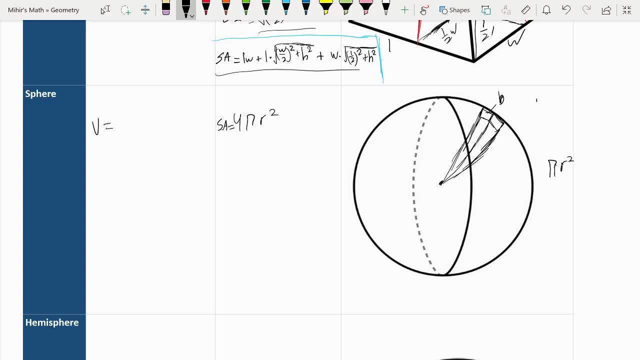 well, if we remember the volume of a cone, that's one-third base times height. But in this case, for these cones, this height here is actually the radius of this cube. If you look at it this height here, I'm going to go in red. 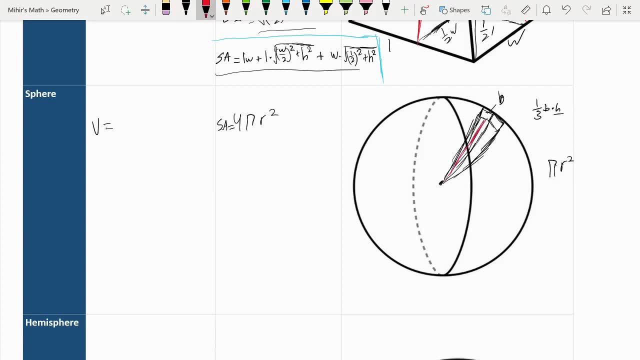 this height is actually just the radius of this cube. It's the radius of the sphere, not cube, sorry. So we can replace this h with. we can replace it with one-third base times r. So if we took all of the bases, 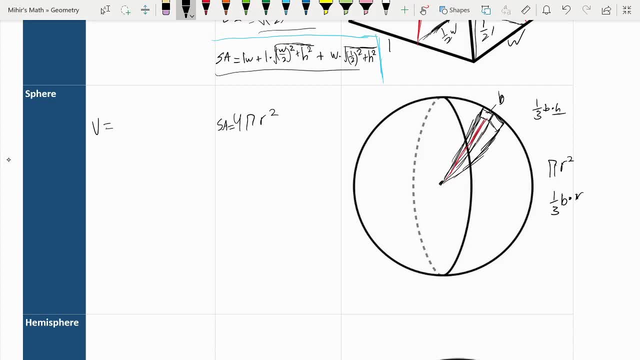 which I'm going to represent as capitalized B, so one-third capitalized B r, with all of these bases being multiplied by one-third in r, what would happen is, since these are so infinitesimally small, these bases here are just actually making up the surface area. 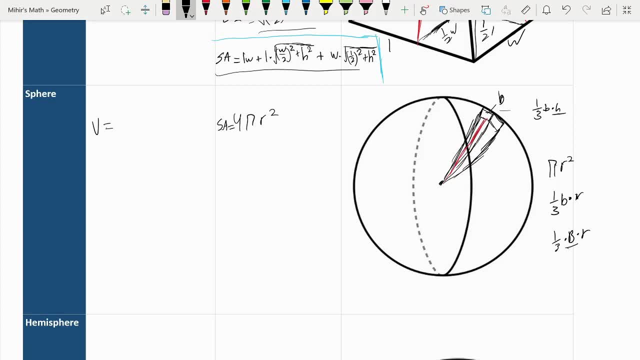 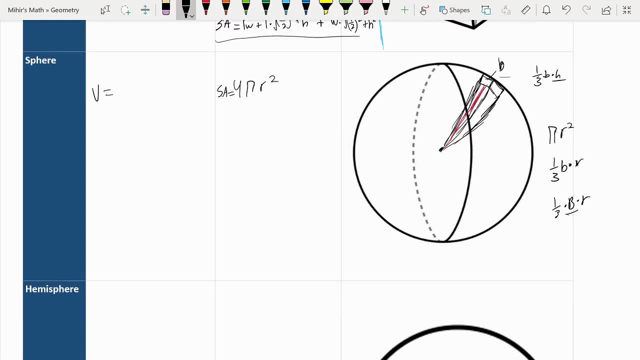 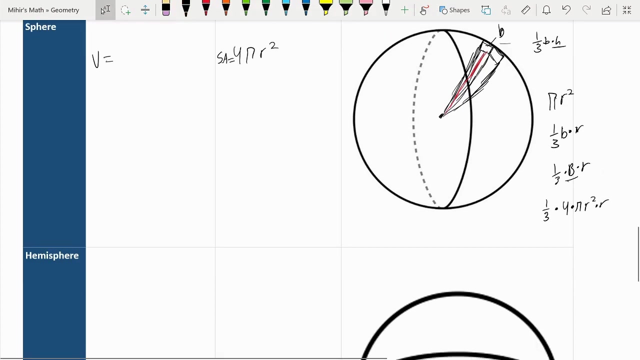 So what we can do is we can replace this base over here, all of these bases together, and we can replace all of those bases together with one-third With one-third times four times pi, r squared times r. So if we were to simplify this, 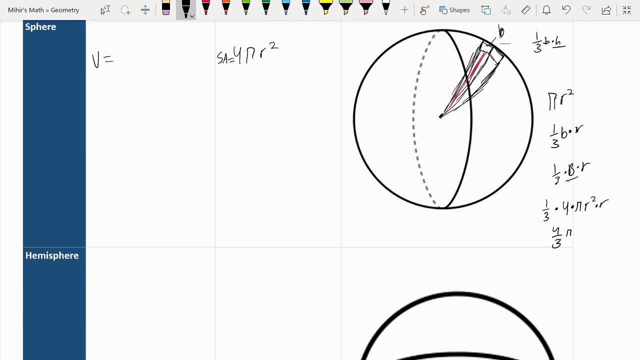 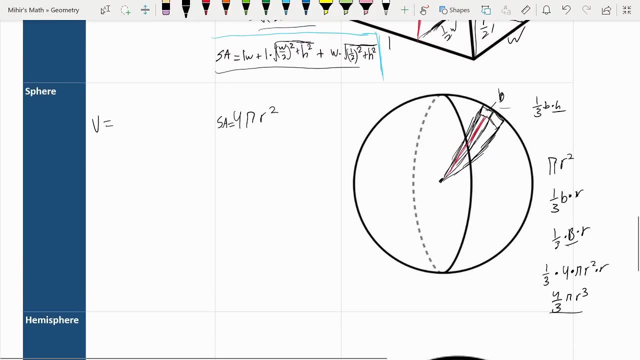 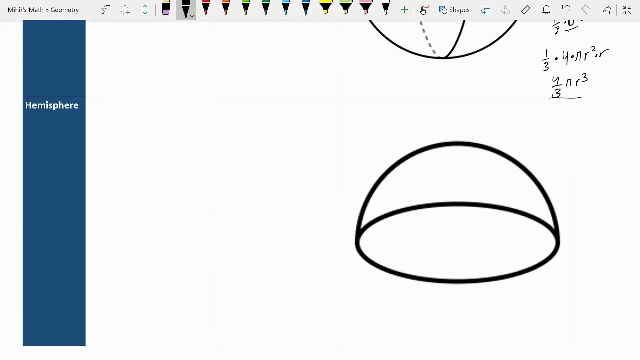 this gets you four-thirds pi r cubed. So that's how you can sort of think your way through that one. So four-thirds pi r squared times r So four-thirds pi r cubed. So the last shape we have is the hemisphere.